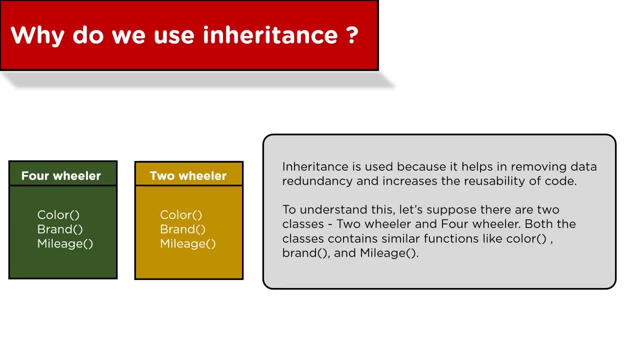 it helps in removing the redundancy. To understand it, let's suppose there are two classes, two-wheeler and four-wheeler. Both of the classes contain similar functions like color, brand and mileage. Now, if we create these classes, we will get the following information. First of all, we 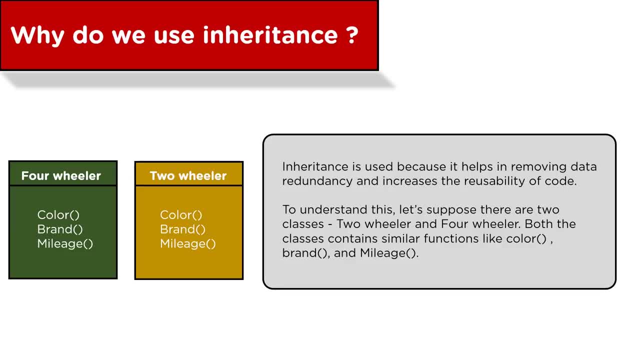 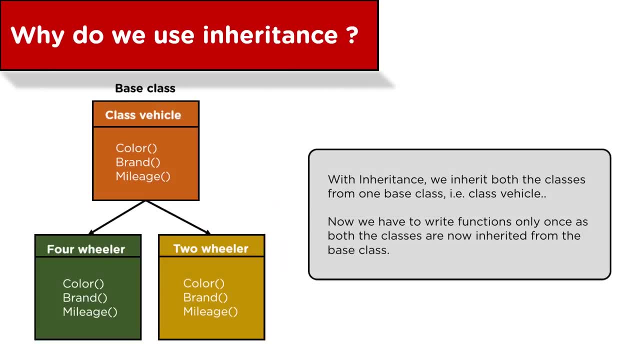 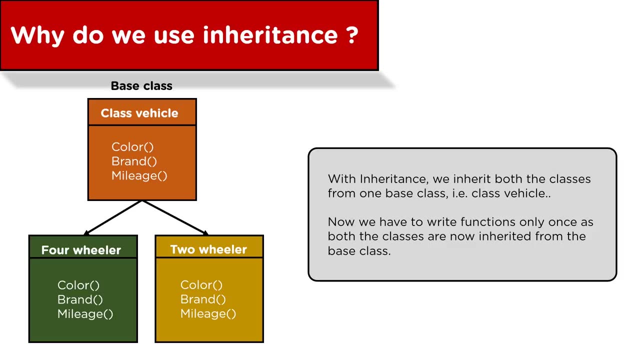 need to create the code of inheritance Loadingopillainserm소�, comparative to code from class to class. So, instead of writing code in both classes, we can use inheritance and create a parent class named classvial, And both the two-wheeler and four-wheeler classes will be inherited. 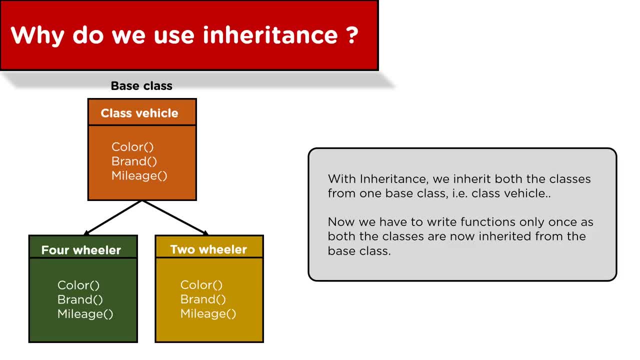 from this parent or base class. Now we have inherited both classes from a base class in inheritance vehicle. now we no longer have to write the code again and again and we can simply write the functions once in the base class, as both of these classes are inherited from the base class vehicle. 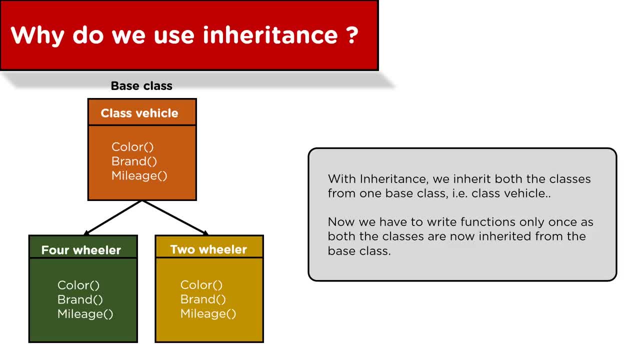 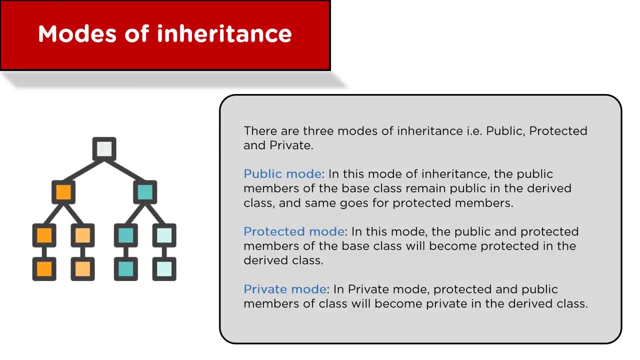 so, as we have understood about inheritance in c++ and why we use inheritance in c++, so now let's go ahead and learn about modes of inheritance. there are three modes of inheritance in c++, that is, public mode, protected mode and private mode of inheritance. so let's start with the public mode. 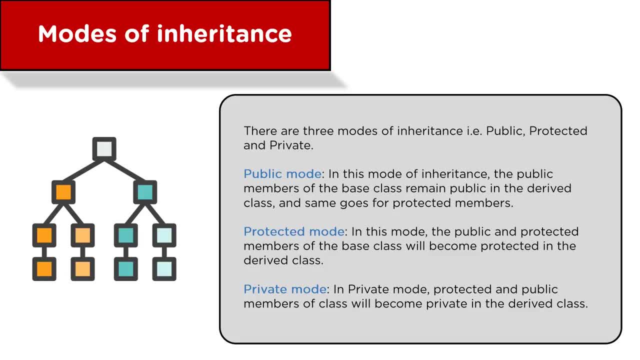 in this mode of inheritance the public members of base class remains public in derived class and same goes for the protected members. that means inside the base class. the class members that are public will remain public in the derived class and similarly, protected class members will remain protected in derived class. now protected mode. in the protected mode, the public. 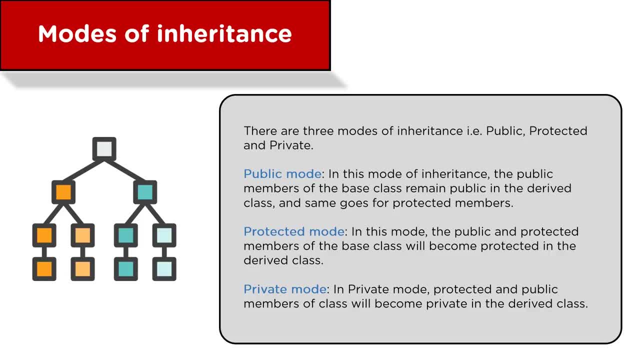 and protected members of the base class will become protected in the derived class. that means the class members which are public or protected in the base class will all become protected in the derived class in the private mode of inheritance. protected and public members of class will become private in the derived class. so now let's go ahead to the types of 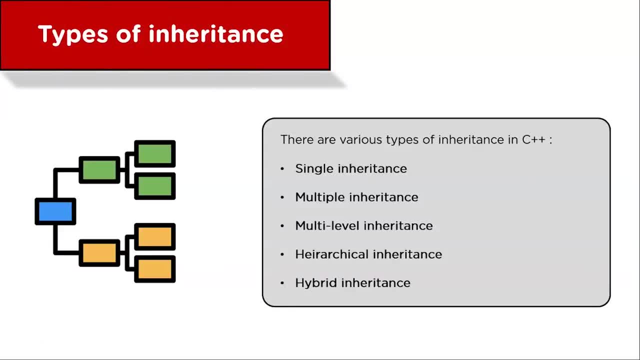 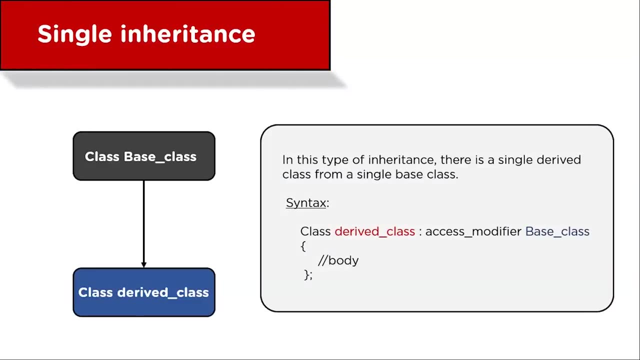 inheritance. so there are various types of inheritance in c++, that is, single inheritance, multiple inheritance, multi-level inheritance, hierarchical inheritance and hybrid inheritance. So let's start with the single inheritance. In this type of inheritance, a single derived class is inherited from the single base class. It allows the derived class to inherit properties. 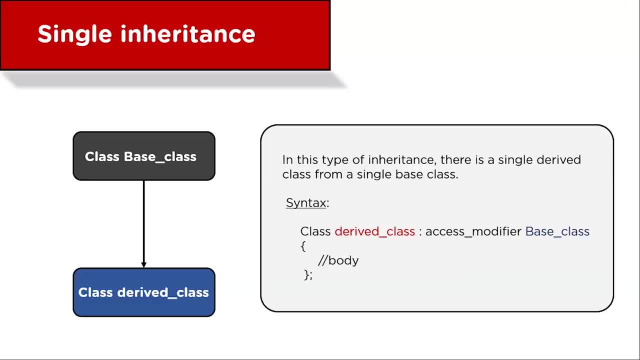 and behavior from the parent class. The derived class objects can access the members of the base class, but the base class objects cannot access the members of the derived class. So now let's have a look at the syntax. As we know, this is single inheritance, so there will be only a single. 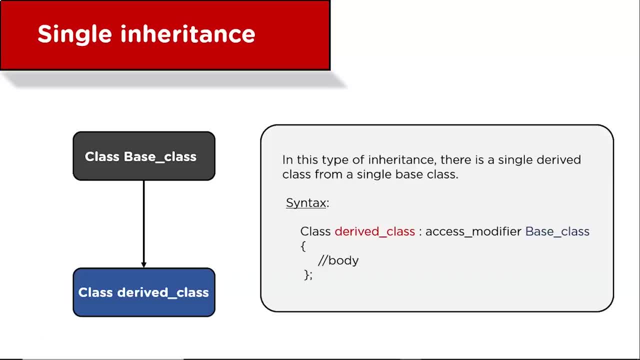 derived class and a single base class, and this is how we derive a child class from a parent class: Class keyword, then the name of the derived class, then the colon operator. after that there is an access modifier with the base class. Now, as we have understood about single inheritance and its 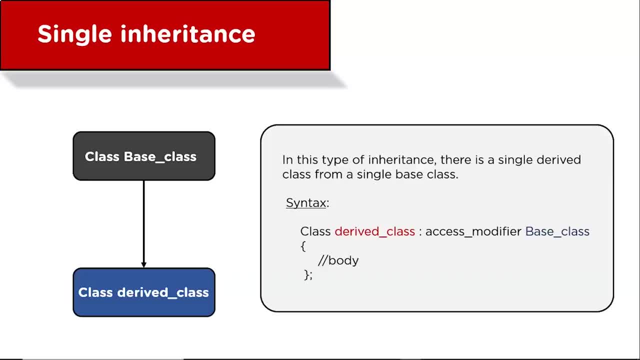 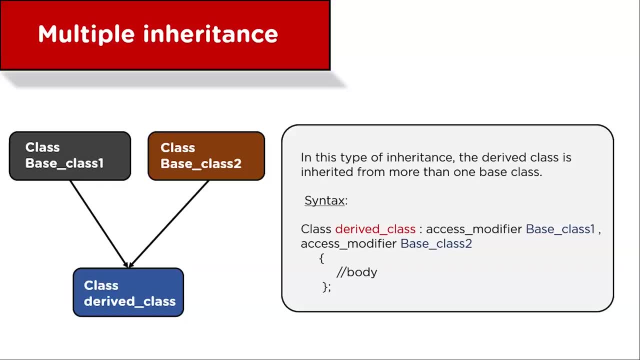 syntax. now let's move on to multiple inheritance. Multiple inheritance: When we have understood about single inheritance and its syntax, let's move on to multiple inheritance. When a class inherits from more than one base class or multiple base classes, then it is known as multiple inheritance. It allows us to inherit properties and characteristics from more than one. 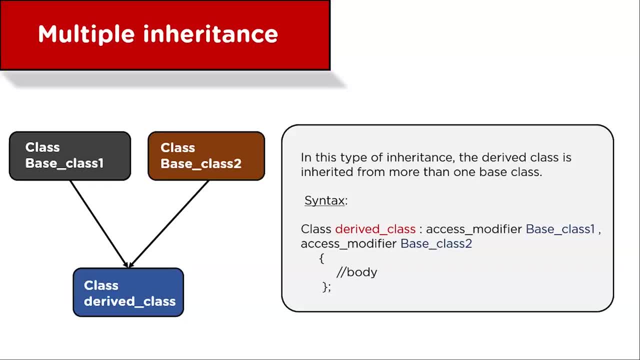 base class. Syntax for multiple inheritance is class keyword with the name of derived class, then the colon operator and access modifier with the name of the base class, separated with comma, and the name of another base class. Here we have shown only two base classes, But we can make more than two base classes depending upon our requirement. 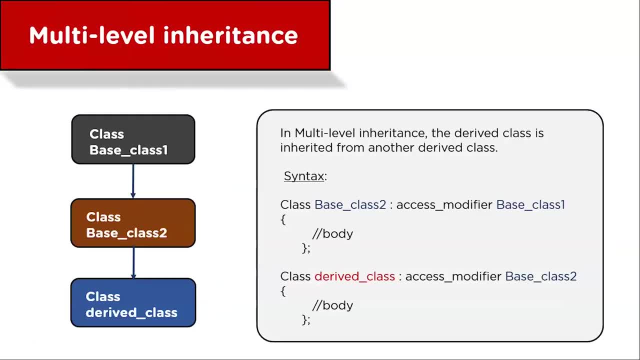 Now coming to multi-level inheritance. In this type of inheritance the derived class is inherited from another derived class. that means when a class extends a class that further extends another class is known as multi-level inheritance. For example, if there are three classes: A, B, C. 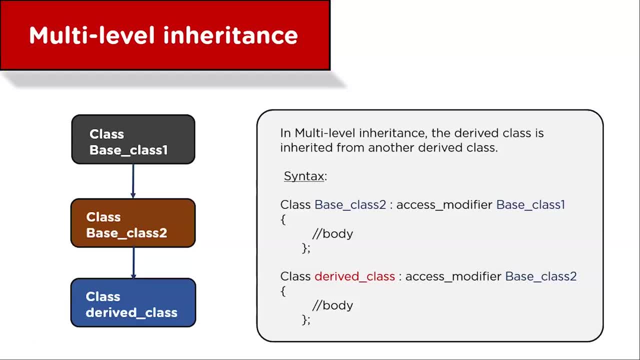 and class C is inherited from class B and class B is inherited from class A, then it can be called as a multi-level inheritance. Syntax of multi-level inheritance is as follows: Base class 2 is derived from base class 1 and the derived class is derived. 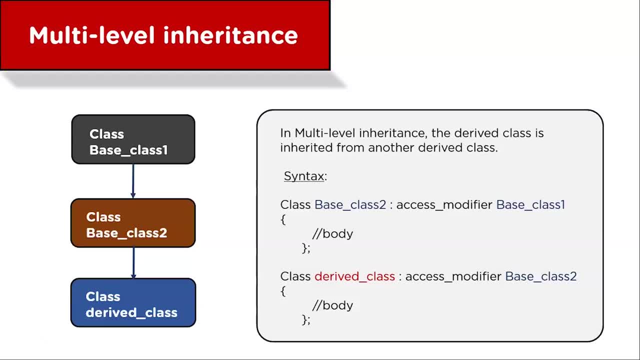 from base class 2.. These base class 1, base class 2 and derived class are just the names, not a syntax. You can write whichever name you want with the class. Now let's learn about hierarchical inheritance In this type of inheritance more than 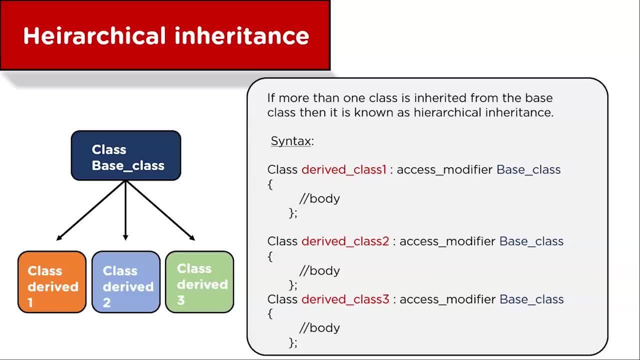 one class is inherited from a single base class, that is, there would be a single base class and multiple derived classes which have the properties and features same as that of the base class. As we can see in the figure and in the syntax, the derived class 1 is derived. 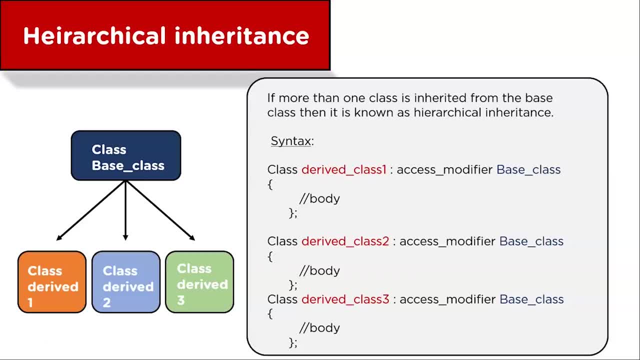 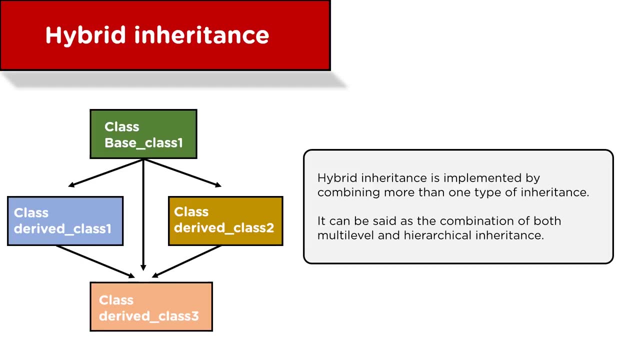 from base class and similarly derived class 2 and derived class 3 are also derived from the base class. So this was hierarchical inheritance and our next type of inheritance would be high-branched inheritance. The hybrid inheritance is the combination of more than one type of inheritance and it can be said: 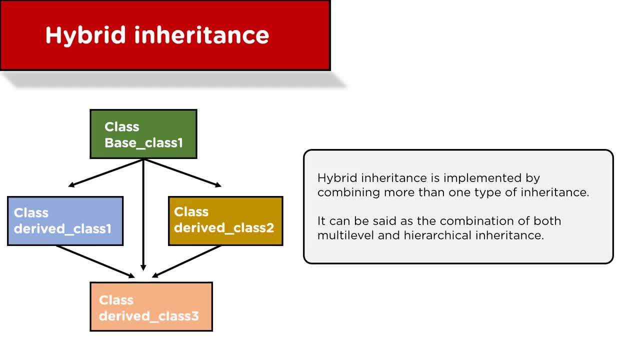 that it is a combination of multi-level and hierarchical inheritance. In the figure we can see the base: class 1 is a parent class of derived class 1 and derived class 1 is the parent class of derived class 3, which makes it multi-level inheritance. But if you 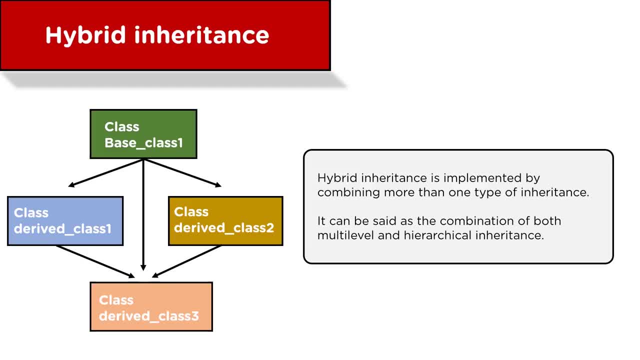 look at it in this way that the base class 1 is the parent class of derived class 1, derived class 2 and derived class 3, then it is hierarchical inheritance, as multiple classes are inherited from a common base class. So we can say it is a combination of more than one type of 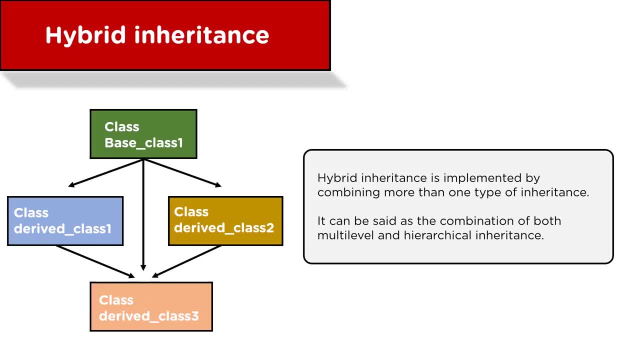 inheritance or a hybrid inheritance. So as you have understood about inheritance in C++, so now let's go to its practical aspect and do some examples on our code editor, that is VS Code. So this is our Visual Studio code and now we will do an example of inheritance. 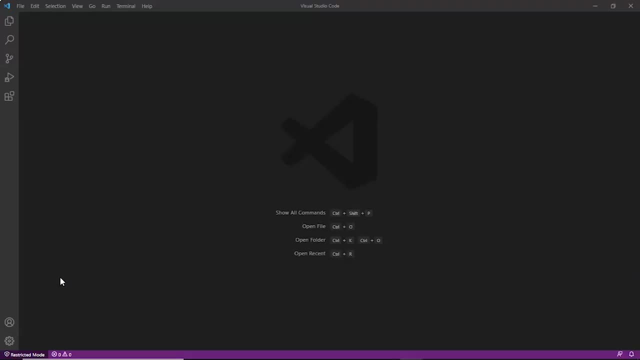 We'll start by doing the single inheritance example, in which we will make a parent class and a child class. And let's start. First of all. we'll create a file and let's name this file as let's name it: inheritcpp. 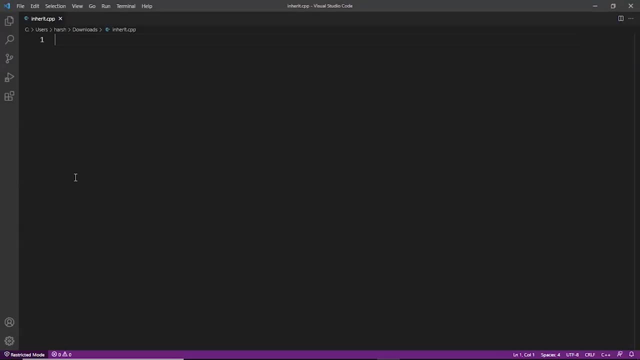 So here we'll do an example in which you will create two classes, a base class in a derived class, and we'll create functions in those classes. like we'll create one function- base class and one function in derived class and using the object of derived. 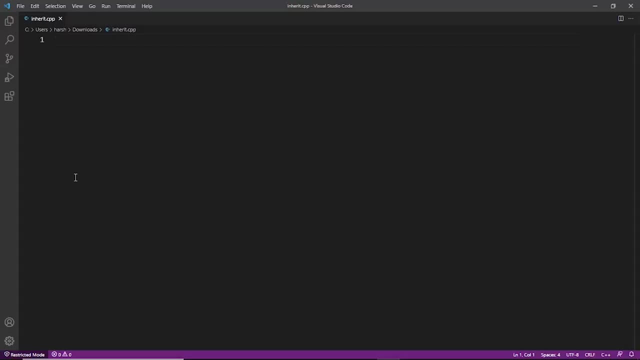 class, we will access the member of parent class or base class. So let's start. First of all, we'll include the header files, hash, include IO stream, Now the namespace standard using namespace std. Now we'll create a base class first, then afterwards we'll create 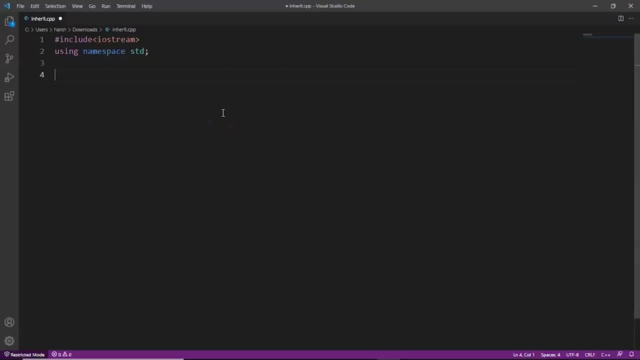 the main function. Alright, so let's create the base class. Let's say the name of the base class or the Parent class would be my rage- And inside this class, let's make this go public. and Now let's create a function. as we have said, drinks, So this is a function. 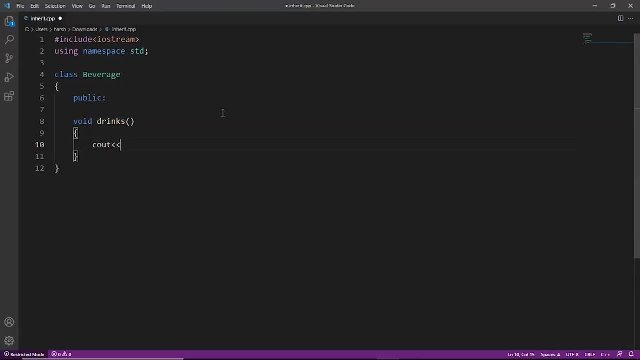 and we will print something inside this function. So let's say we are printing: all rings are available, All trains are available Now. right handle Now will use semicolon in the end of the class. so this is a base class and we 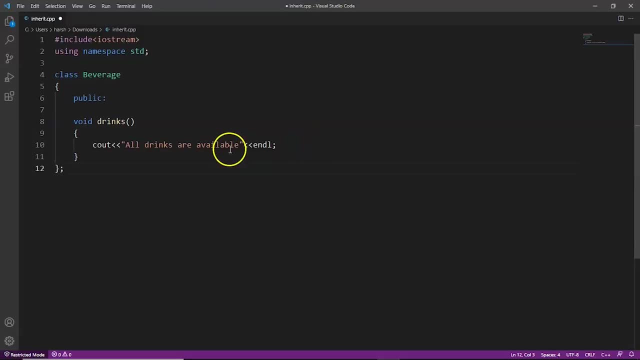 have created a function- drinks- and we have printed a message- all drinks are available, all right. now we will create another class, which is derived class or child class. we will write class: coffee is the name of the derived class. use the colon operator public access specifier and the name of the base class, that is. 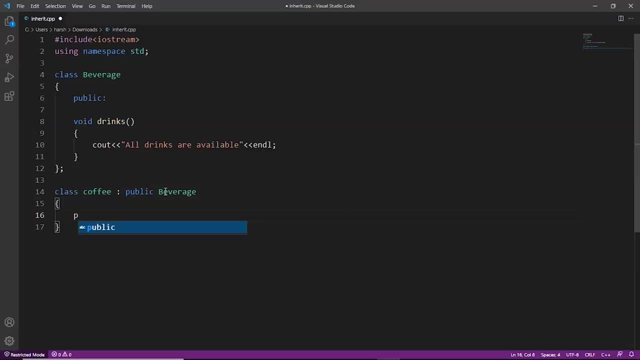 beverage. all right, now we'll write public access specifier inside this class and we will create a function in this class also, like, let's say, the name of the function would be mocha- it is a kind of a coffee, so mocha, and we will print that mocha tastes good, tastes the best. I would say: okay, now let's use the. 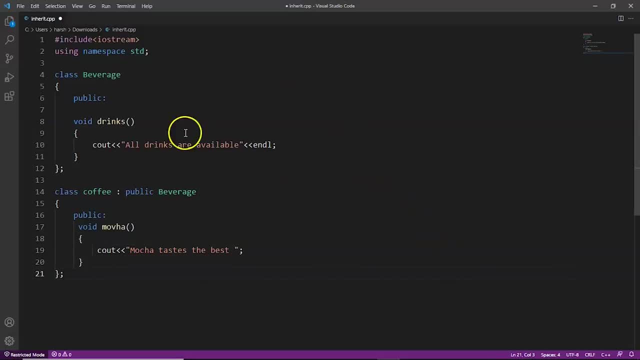 colon operator in the end of the class. so we here we have the name of the beverage and we will write public access specifier inside this class and we will create a function in this class also, like let's: here we have created the parent class or base class and this derived class or 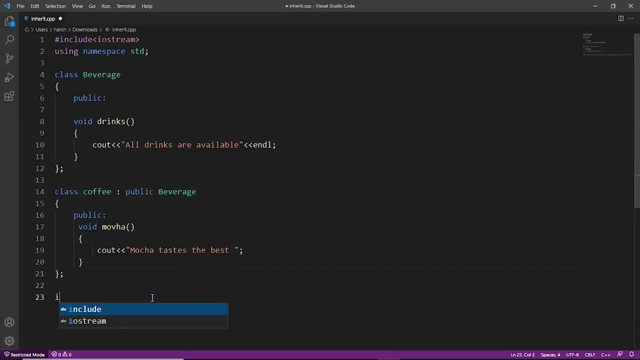 child class. so now we will create the main function, we will do the calling. so now we will create the object of child class. so our child class is coffee and now we will create the object. that is, see the name of the class and the object. okay, now we will use the object with dot operator and call this function, that is. 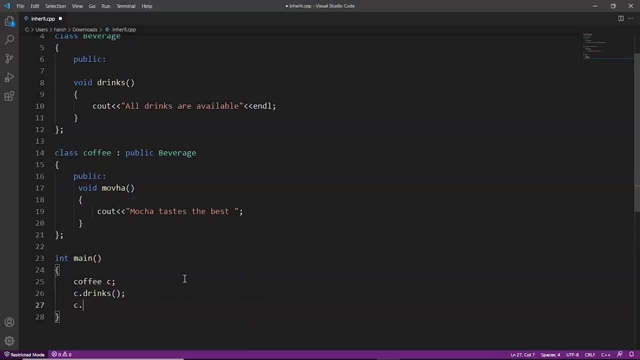 drink. and now, using the same object, we'll call the mocha. the spelling is wrong. yeah, now it is right: mocha. so, using the object of child class, here we are calling the drinks function, which is of the parent class. so let's see if it works. 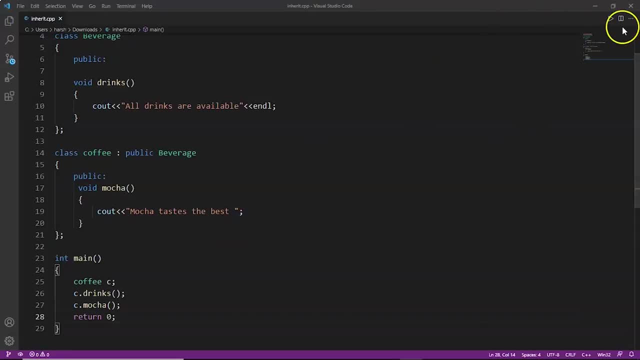 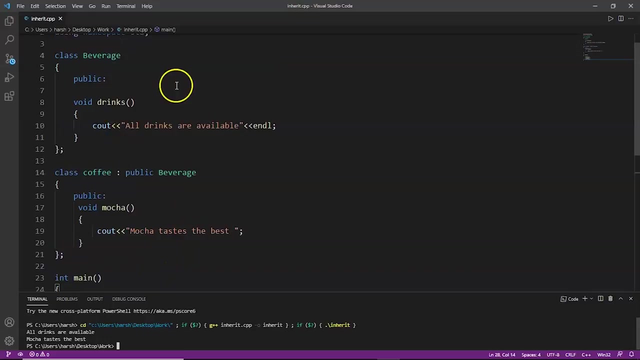 or not, let's save it and now run it. as you can see, all drinks are available and mocha tastes the best, morning coffee tastes the best. Both of these are getting printed. That means the object of child class is able to access the member of the parent class. 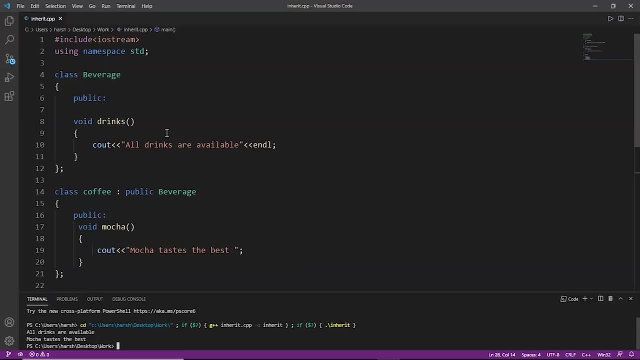 So this is inheritance, when the child class acquires or inherits the behavior or characteristics from a parent class or access the members of the parent class. This is an example of single inheritance. So now let's do another example of multiple inheritance. So let's create a new file and name it as inherit two dot CPP. 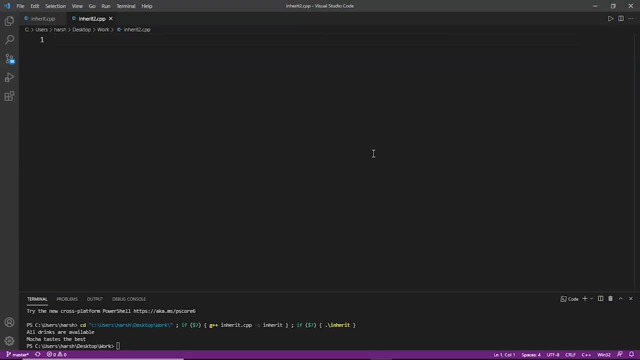 All right. Now here we'll do an example of multiple inheritance, in which we will create two base classes and a derived class, As we know that in multiple inheritance there are more than one base classes to a single derived class. So let's start. 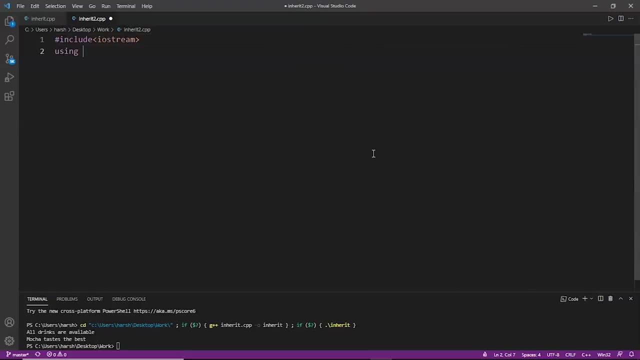 First of all, we'll include the header file. Now we'll use the namespace standard And now we will create a new file. We will create a class, that is the base class, and we'll name it as party, So class party. inside this base class, we will first of all declare the public scope. 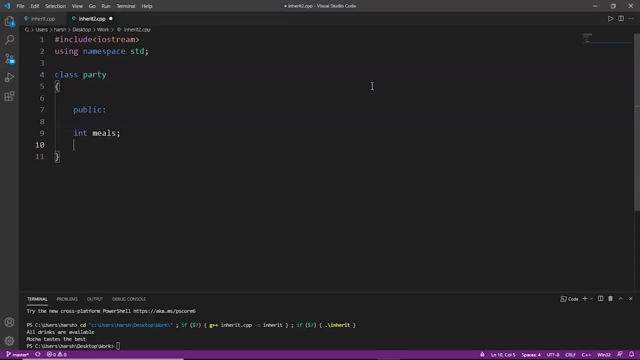 And now we will declare a variable, let's say meals. So now we will create a function and in this function we will take the input from the user about the number of meals to enter the number of meals. So let's start void food. 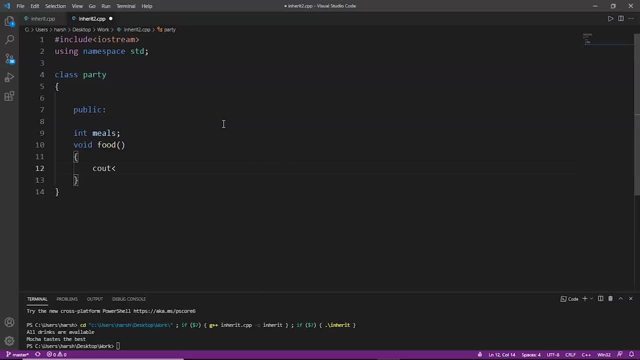 This is the function name And first of all, we'll display the message saying that: enter: number of meals. All right, Now we will take the input and meals is the variable. Now we will use the semicolon at the end of this class. 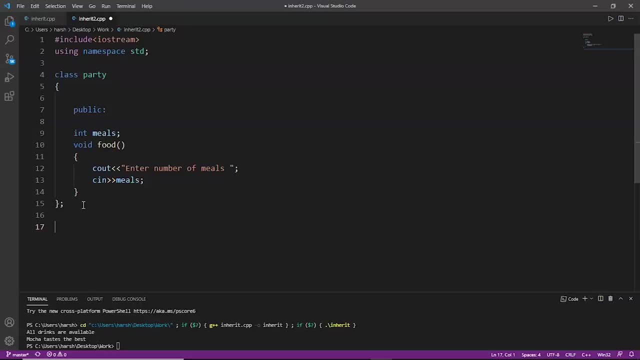 So in this function we are taking the input of the number of meals. now in this, in the other class, That is, another base class, We will take the input of number of drinks from the users And then in the derived class figure out the total bill of the party. 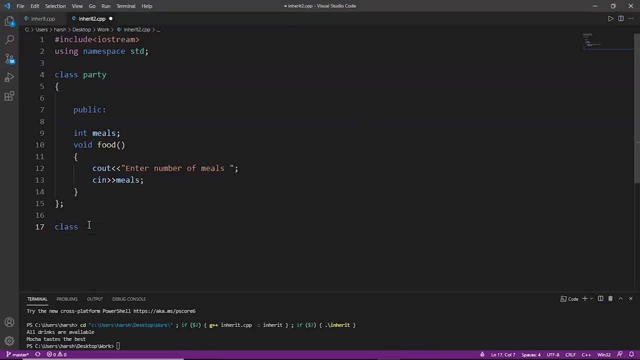 All right, Now we will create another base class, that is, drinks, not drinks drinks. All right, Now we'll write the public scope And similarly, we'll create or declare another variable, drink, And Then now we will create a function. 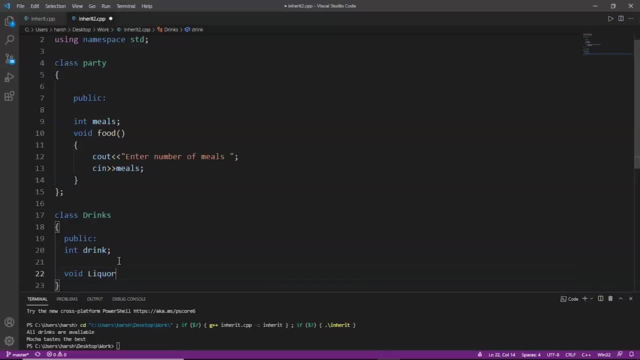 Let's say the name of the function is liquor. All right, Now, inside this function we will take the input from the user regarding the number of drinks, So we'll display the message and the number of drinks, So the user will enter the total number of drinks used in the party or consumed in the 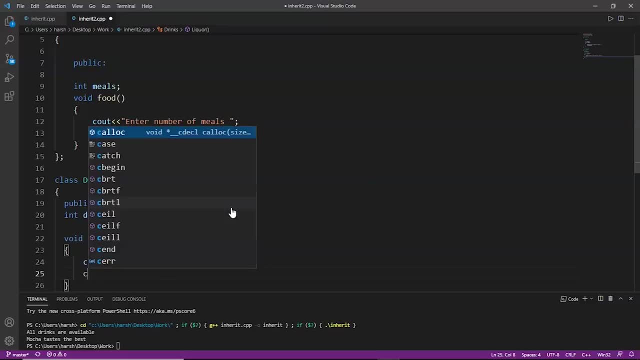 party. Similarly goes for the meals, No. So we take the input and will write: drink, drink. All right, Now we have created this liquor function. Now we will use a semicolon at the end of the class where we have created both the base. 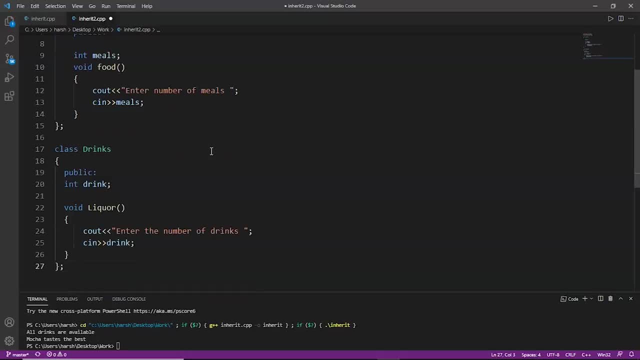 classes, that is, class party and class drinks. Now we have to create the derived class. So this is an example of multiple inheritance. So we will create the derived class And use the Column operator. Now we will write the public specifier and the name of the base class for space class. 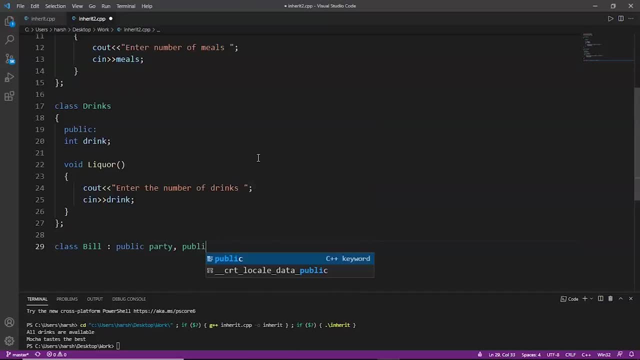 would be party separated with comma. The second base class would be drinks. All right, So this is how we can do that. Now, inside this class, we will first of all create three variables. let's say in total, meals In total. 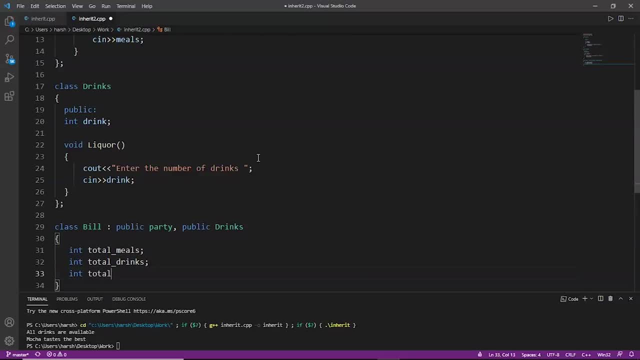 Drinks and in total bill, because in the end we have to find out the total bill. All right, Now, inside the public school, we will create a function name as total. Now, inside this total function, we'll write the logic to calculate the total bill. 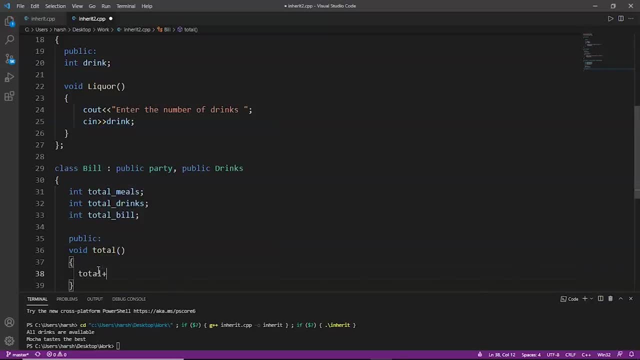 So what we'll do is first of all write the total meal- Total meals Equals Meals- Into the price of a single meal. Let's say the price of a single meal is 90. So the total product would be stored in total meals. 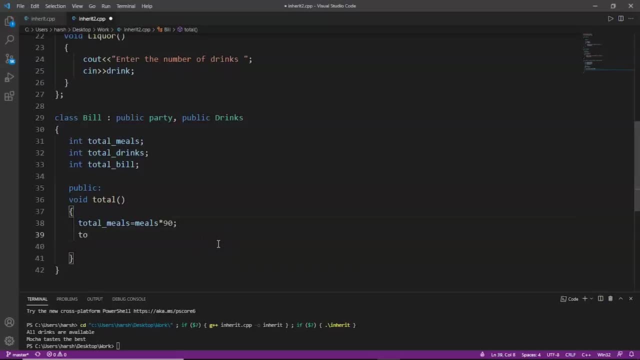 All right, Now we'll do same for total drinks. Total drinks not Frank's girls drink into. Let's say, the price of a single drink is 60.. Yes, All right Now. after that we have to compute Or calculate the total bill. 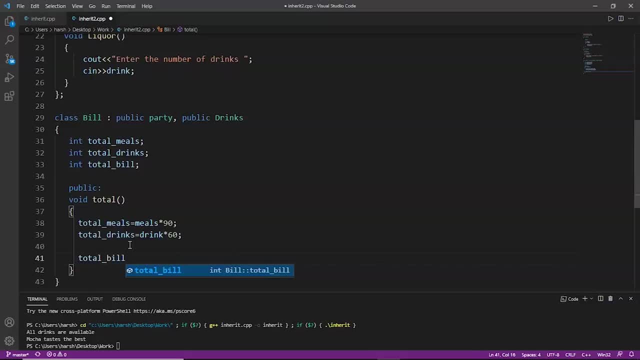 Total bill would be the addition of both of these: total meals plus total drinks. So we'll simply do the addition over here: Total drinks. So once it's calculated, we'll simply display a message saying that the total bill for the party total bill for the party is and we'll write the variable that is total bill where. 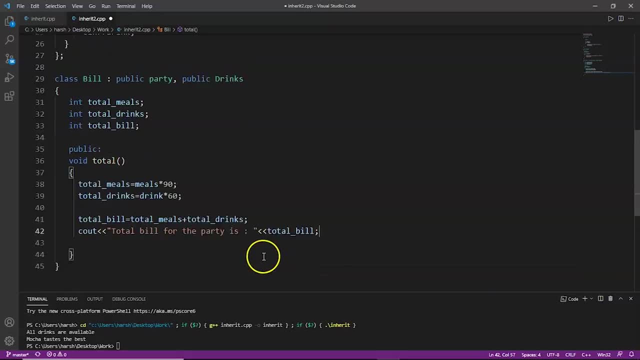 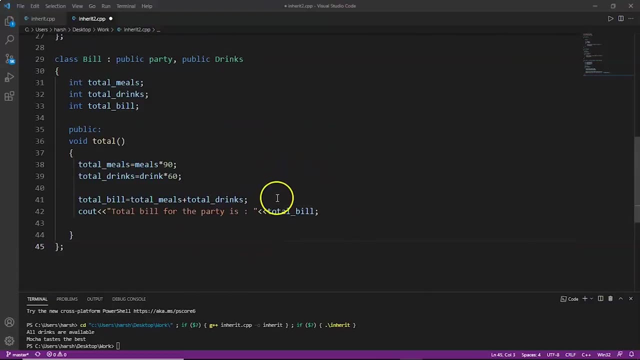 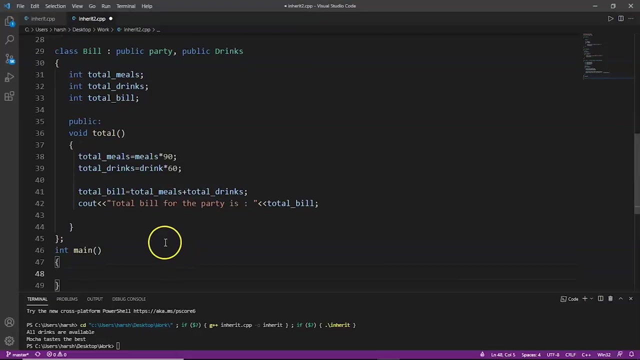 the total Bill. So this is actually getting stored All right. After this we'll use the semi-colon, So this is the derived class. here We have calculated the total money spent in the party. So now we have to write the main function where it all started, inside the main function. 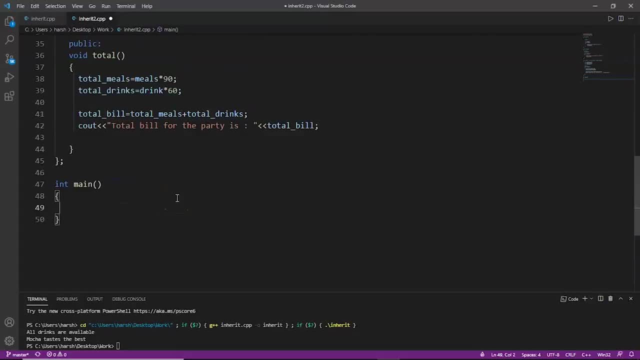 First of all we will create the object of child class. So we know that our child class or the derived class is bill. So bill is the derived class and B would be the object. So using this B, we will first of all call a function, that is food function. 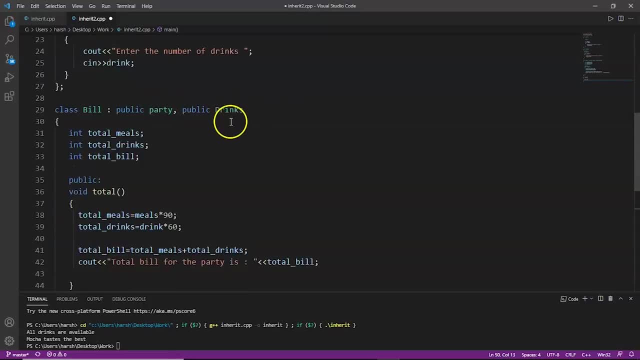 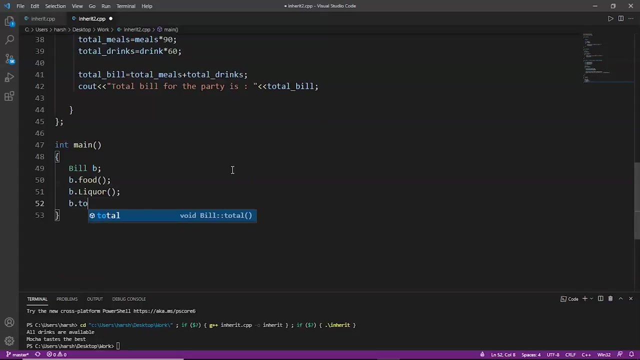 So by calling this, we will take the input of number of meals. Now we will call another function named liquor. All right, Using this function, calling this function, we'll take the number of drinks from the user. Now we will call this total function. 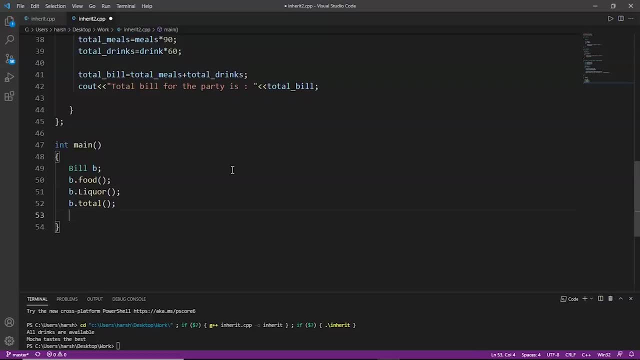 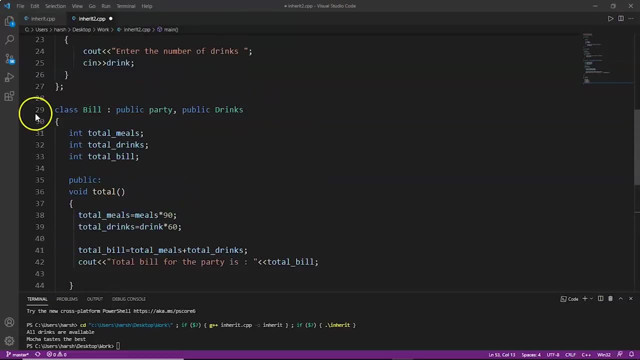 So this will calculate the total money spent in the party, And after that, let's say, return zero. We are calling all of these functions using the object of derived class, And this is where multiple inheritance is going on. So let's see whether it works or not. 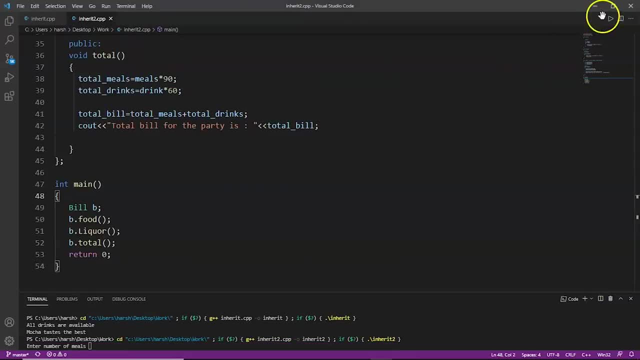 We'll save it and we'll try to run this. Enter number of meals, as we can see. Enter number of meals. Let's say the number of meals would be 20.. It was a short party. Then enter number of drinks: 17 would be. 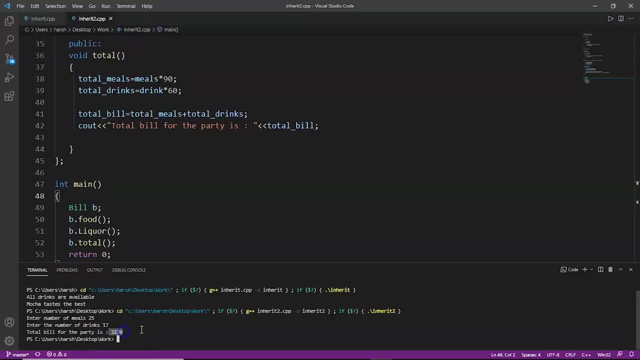 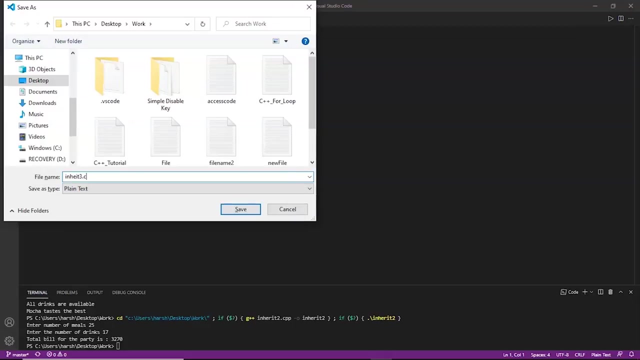 So our total bill for the party is 320.. 270, which is the correct answer. So this is how we can do multiple inheritance, And this is a fine example of multiple inheritance. Now let's do another example. Let's name this one as inherit three dot CPP. 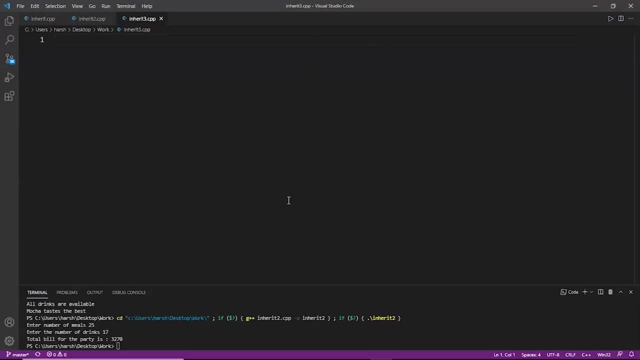 All right. So here we will do an example of multilevel inheritance. And we know that in multilevel inheritance a single derived class is inherited from another derived class. Or in other words we can say: A class extends a class, which further extends another class. 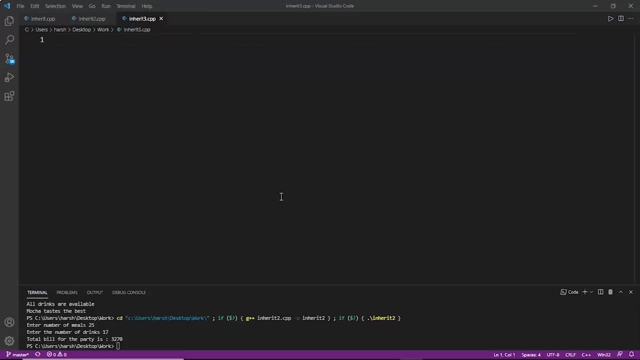 Then it is called a multilevel inheritance, as the name suggests. So we'll do an example of that. In this example we will calculate the marks of a student scored by him in three subjects. We will calculate the total marks scored by him using multilevel inheritance. 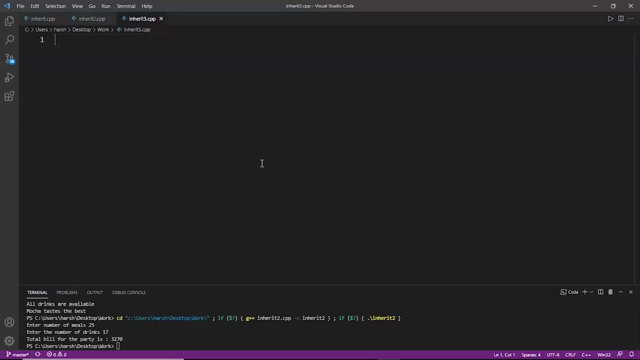 So let's do this. So first of all, we will include the header file as include our stream, then we will write the namespace. Now we will create the class base class chemistry. All right, In this class, first of all, we will make the public school and marks one. 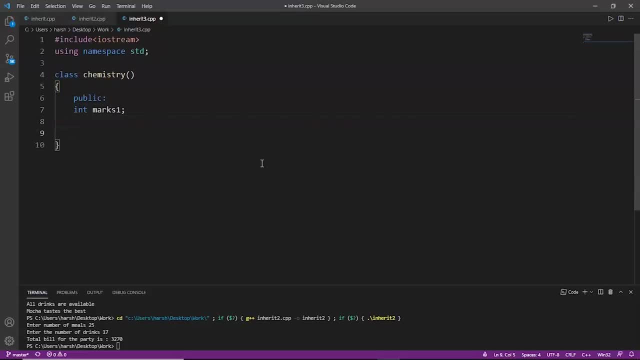 So here we'll take the input of marks scored by that particular child in this chemistry subject. So we'll create the chemistry function, white chemistry, which is of same name as that of class, So let's say chemistry marks. All right, Now we will display the marks scored in chemistry and the marks scored in chemistry spelling. 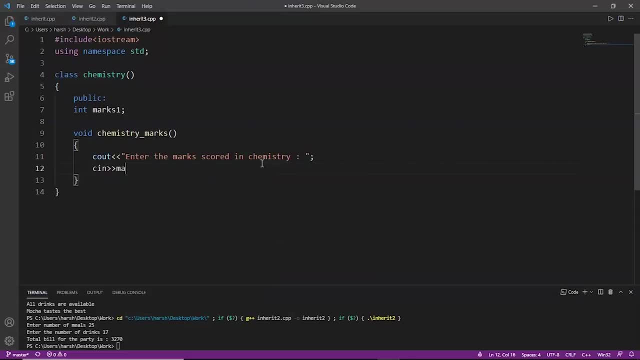 is wrong. Okay, Now we'll take the input marks one, So the student will enter the marks. after that Let's put semi-colon in the end. Now we'll create another class named physics, which is inherited From chemistry class, that is, chemistry classes. it's BS class, chemistry. 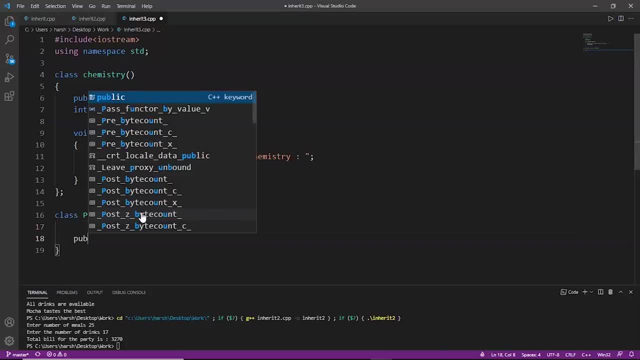 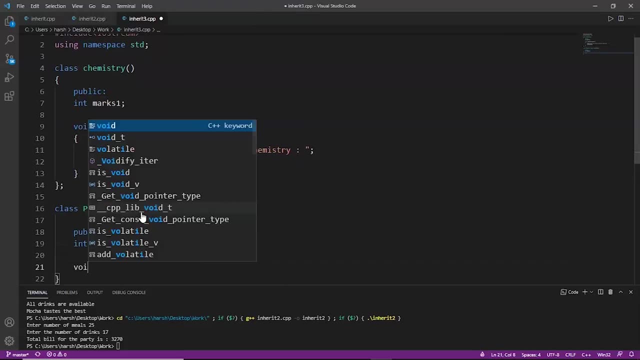 All right. So in this class we will do the same public and marks to marks. to now we'll write void physics marks. We'll do the same as we have done in the previous class, So now we will display a message saying that. 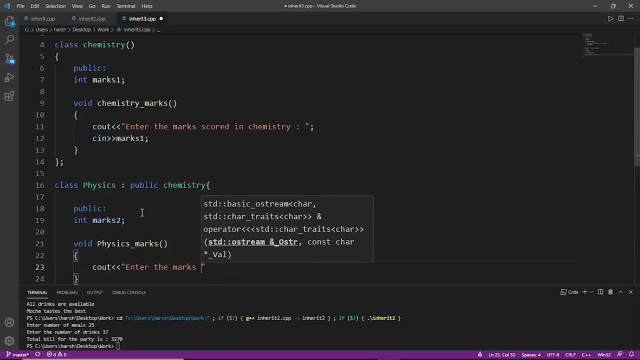 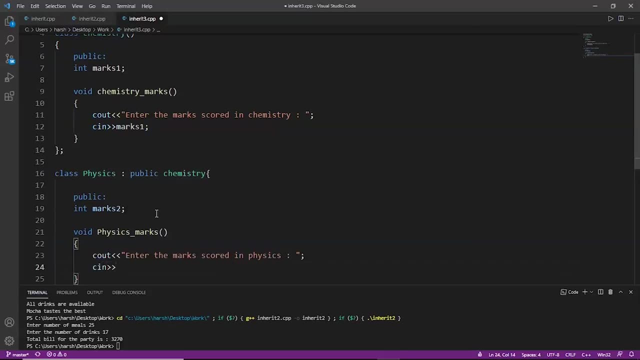 Enter the mark, Enter the mark, Enter the marks in physics to write. Now it will take the input c in Mark stew. All right, So now we'll put semi-colon in the end of this class as well. So now we know that this physics class is is inherited from this chemistry class. 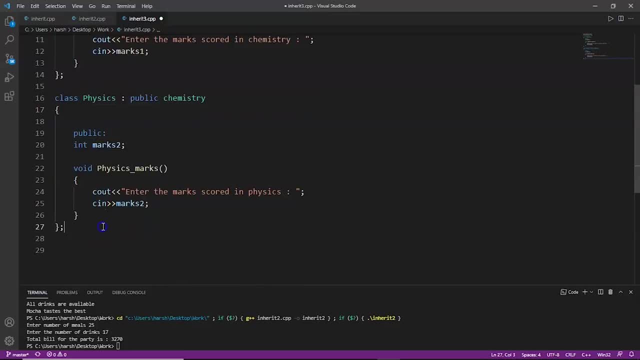 That is, the cluster class, is the best class of physics class. Now we do same for mass, like class mats, Which is inherited from these chemistry class, like lots of those idol, which is in the base class of the physics class. Now we'll do the same for the mats, like class mats, which is inherited03 is the base class. 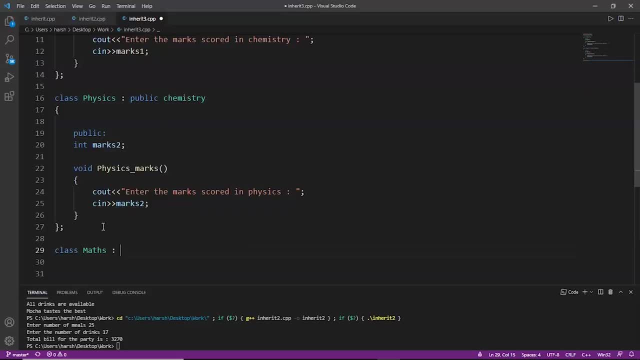 class, which is inherited from the physics class. we will write physics inside this class as well. we'll do the same and, as you can see, this physics class is the base class of maths and the base class of physics class is chemistry, so this is a multi-level inheritance. so in this class we'll 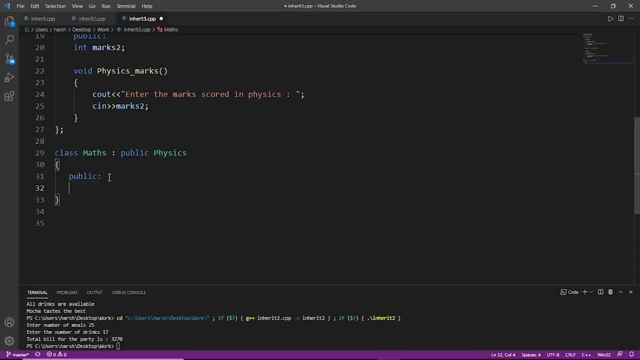 do the same: public scope. and now, after public scope, int marks. three is the variable we have declared, and we will declare another variable in this one, like total, because we have to find out the total marks. now, function maths marks. inside this one, we will display the message that enter. 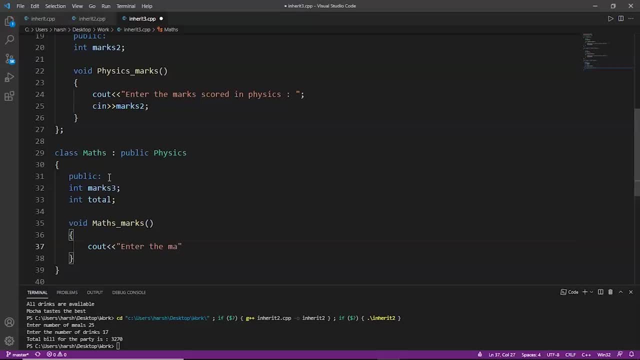 the marks. yeah, enter the marks scored in. you match all. right. now we'll take the input- marks 3- and we'll write the semicolon in the end. so here we have created all of these three classes, which is of multi-level inheritance. as you can see, we have taken the input from the user of its maths, physics and chemistry marks. now we'll do the 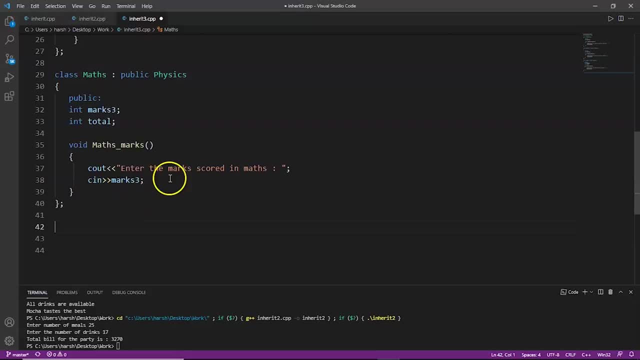 total. so we have to do the total inside this class only, so the name would be result function, and so the total fun variable that we have declared is equal to marks 1, marks 2 plus marks 3. so physics commission, maths marks, we will add all of them and then we will display the total. all right, now this. 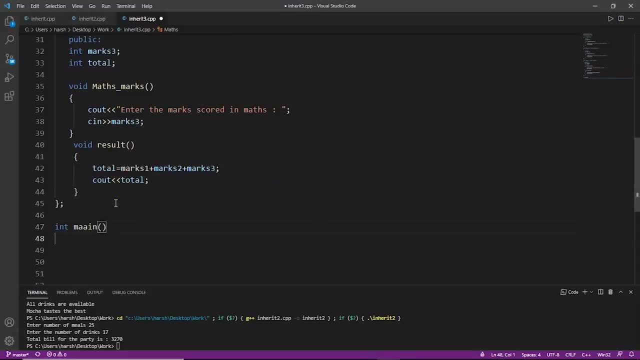 is done. now we have to go to the main function. now, first of all, we will create the object of child class maths. once this object is created now we can call the functions, as it can access the base classes. so chemistry marks first of all, then mphysics marks, mmaths marks and then the total. 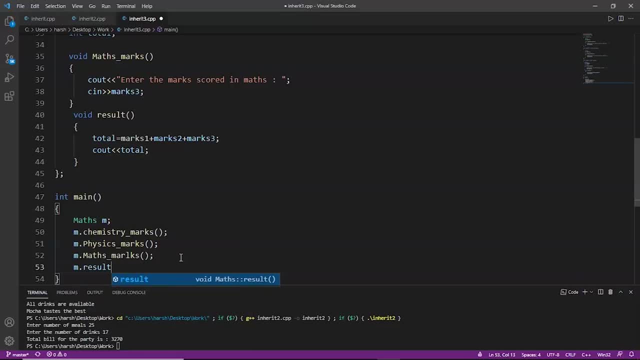 that is result, is the result function and dot. it is right. then we write return zero, so return zero. so here, first of all, mchemistry marks will call this function in the chemistry class, so the user will enter the marks code by him in chemistry. then this will call physics marks, so the user 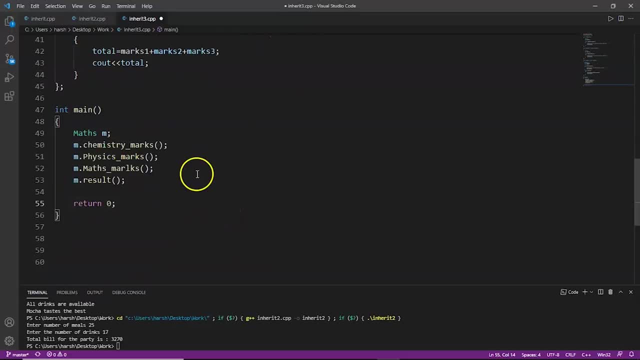 will enter the marks code by him in physics subject. then, similarly, we will match marks. they will enter the marks of max. then we will call the result function. we will do the total of all the marks code by the student, we will do the total and then we will display that total. so pretty much. 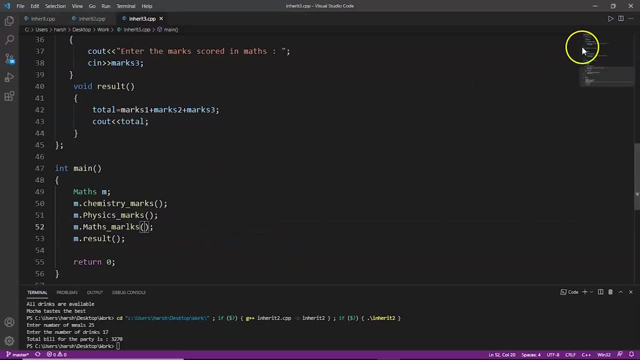 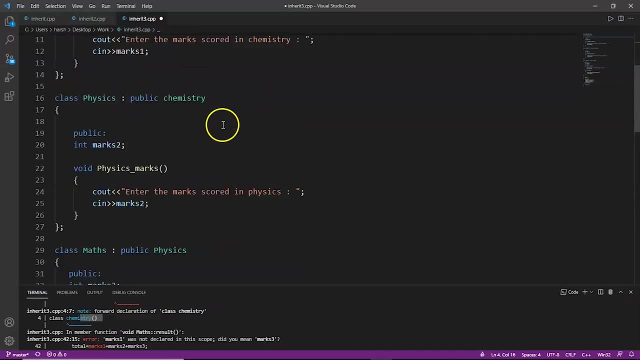 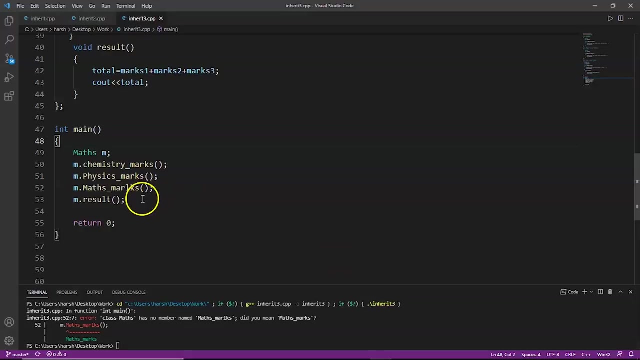 it's done. now we can save it. and now let's try to run this one. there are some errors- all right, that's a silly one by mistake. we have done this. all right, now let's save it and run it again. hope it works now. yeah, another error marks. now let's try again.